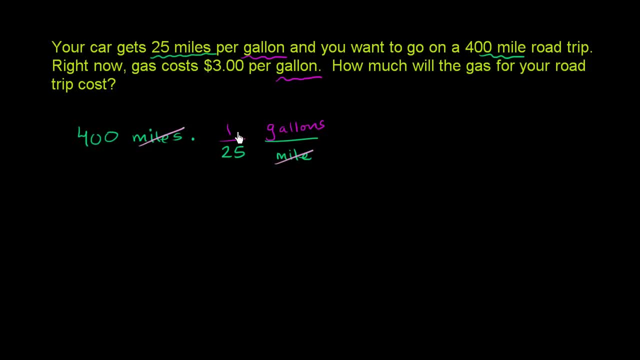 Miles cancel out with miles, And then I have 400 times 1 over 25 gallons, which is the same thing as 400 divided by 25 gallons. So this is equal to 400 over 25.. Which is the same thing as 400 divided by 25 is equal to 16 gallons. 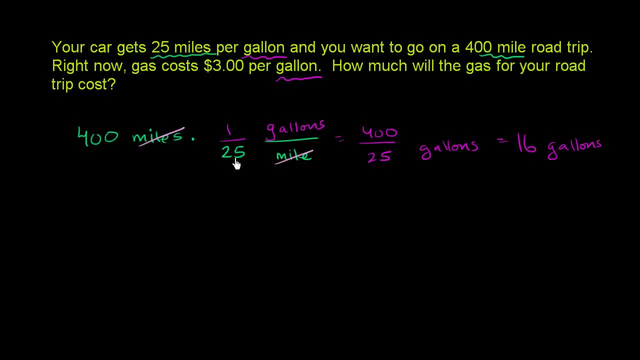 Now, it's always important to do a reality check here, not just to try to blindly cancel out units. Does this actually make sense, that 16 is a much lower number than 400?? Well, sure it does. And actually, if you have any experience filling up a car, 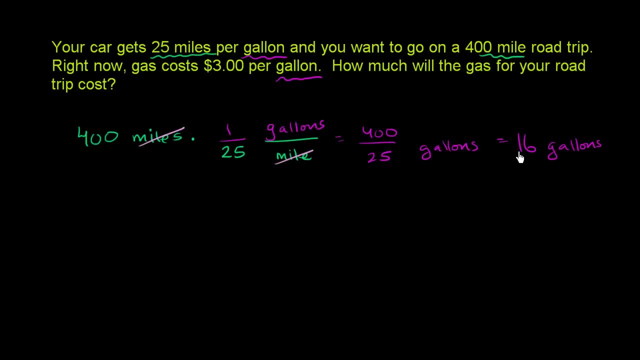 you would sense that. OK, well, that's about the size. on around 16 gallons A car tends to go 300 or 400 miles if it gets pretty good fuel mileage. So that just makes sense from experience And it also makes sense based on how it's stated. 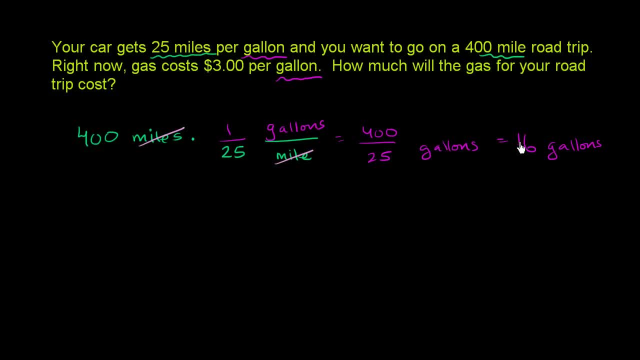 You get 25 miles per gallon, So you're going to need fewer gallons than you're going to need miles. So this all seems to make sense so far, But we haven't answered their question. They want to know how much will my trip cost? 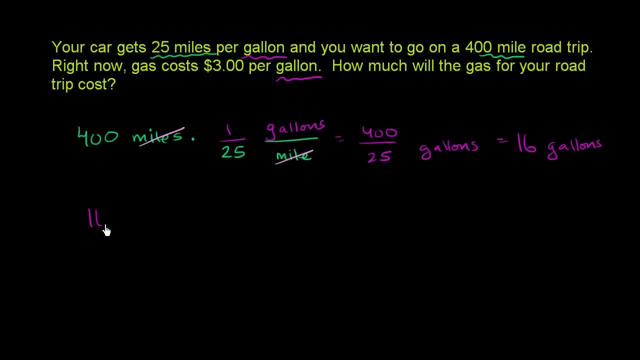 Right now we've just figured out how much fuel we're going to use. So then we could take our 16 gallons And to figure out the dollar cost, we're going to multiply it by dollars per gallon, or gallons per dollar. Well, if we're thinking just about unit conversion, 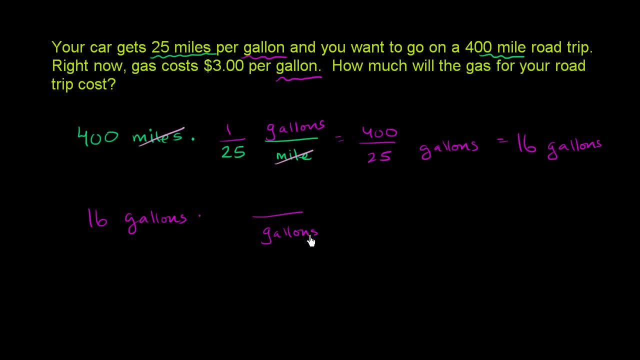 we want to multiply times the dollars per gallon. So I could write it like this: I could write it like dollars per gallon. Actually, let me just write out the word dollar: Dollars per gallon. The units will cancel out And it also makes sense. 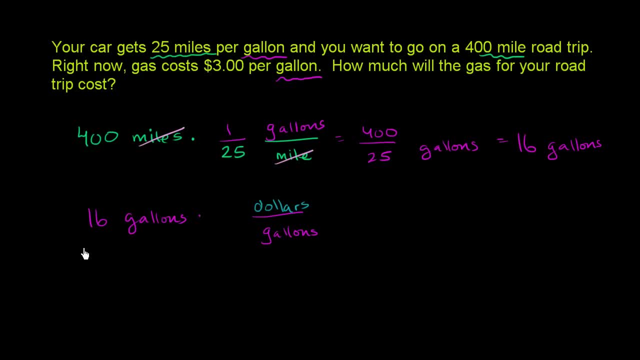 Whatever number of dollars per gallon, I multiply it, times the number of gallons, And that's going to tell me how much it's going to cost. This happens at the fuel pump every day. Hey, it's $3 per gallon. I'm going to fill up 16 gallons. 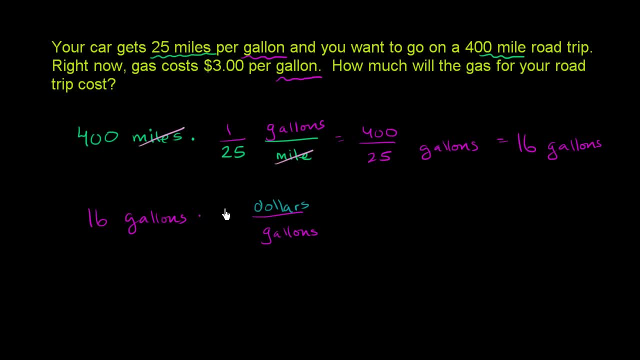 Hey, 3 times 16.. So let's do that. So it's $3 per gallon. We see the gallons cancel out And we are left with $16 times 3, which is the same thing as $48. And we are done. 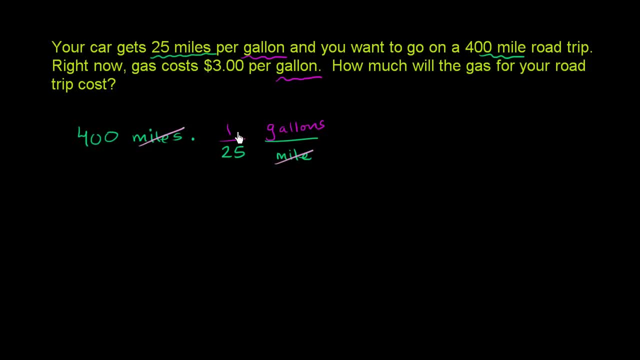 Miles cancel out with miles, And then I have 400 times 1 over 25 gallons, which is the same thing as 400 divided by 25 gallons. So this is equal to 400 over 25.. Which is the same thing as 400 divided by 25 is equal to 16 gallons. 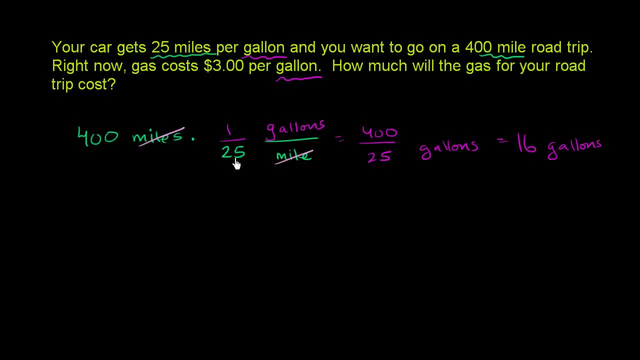 Now, it's always important to do a reality check here, not just to try to blindly cancel out units. Does this actually make sense, that 16 is a much lower number than 400?? Well, sure it does. And actually, if you have any experience filling up a car, 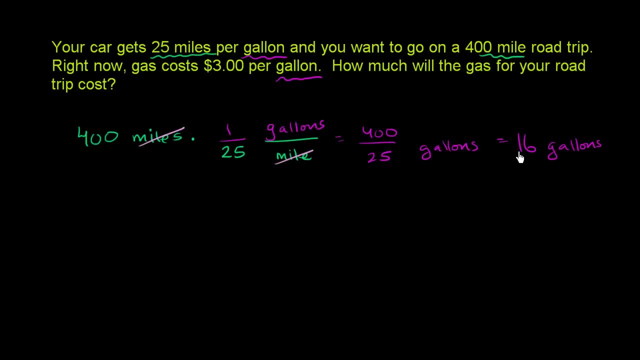 you would sense that. OK, well, that's about the size. on around 16 gallons A car tends to go 300 or 400 miles if it gets pretty good fuel mileage. So that just makes sense from experience And it also makes sense based on how it's stated. 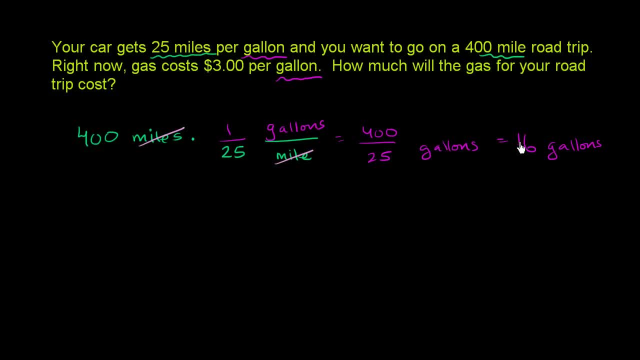 You get 25 miles per gallon, So you're going to need fewer gallons than you're going to need miles. So this all seems to make sense so far, But we haven't answered their question. They want to know how much will my trip cost? 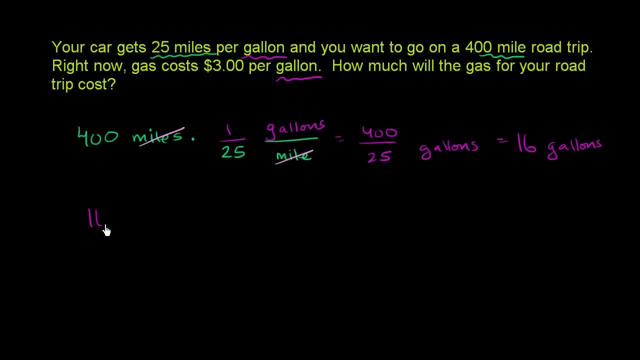 Right now we've just figured out how much fuel we're going to use. So then we could take our 16 gallons And to figure out the dollar cost, we're going to multiply it by dollars per gallon, or gallons per dollar. Well, if we're thinking just about unit conversion, 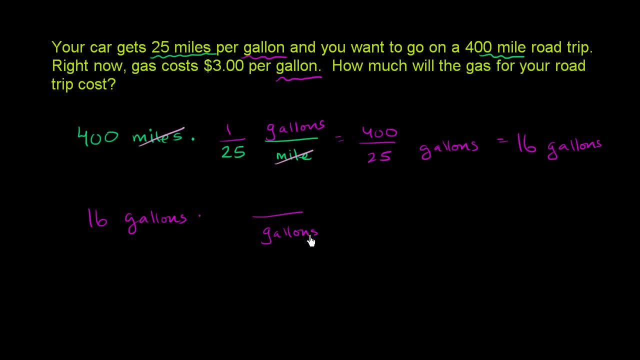 we want to multiply times the dollars per gallon. So I could write it like this: I could write it like dollars per gallon. Actually, let me just write out the word dollar: Dollars per gallon. The units will cancel out And it also makes sense. 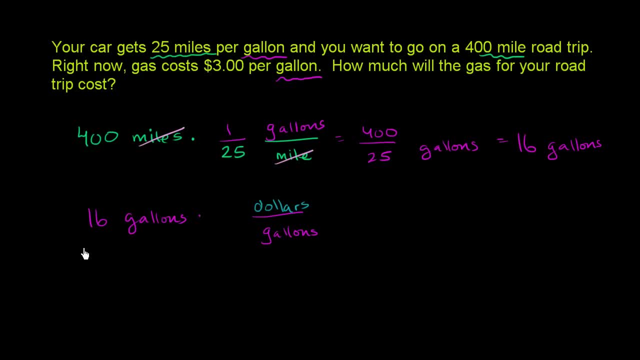 Whatever number of dollars per gallon, I multiply it, times the number of gallons, And that's going to tell me how much it's going to cost. This happens at the fuel pump every day. Hey, it's $3 per gallon. I'm going to fill up 16 gallons. 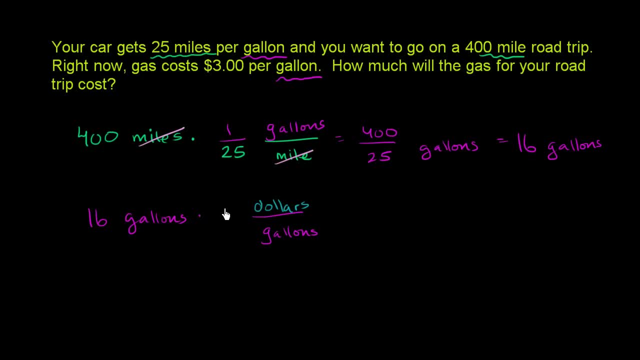 Hey, 3 times 16.. So let's do that. So it's $3 per gallon. We see the gallons cancel out And we are left with $16 times 3, which is the same thing as $48. And we are done.